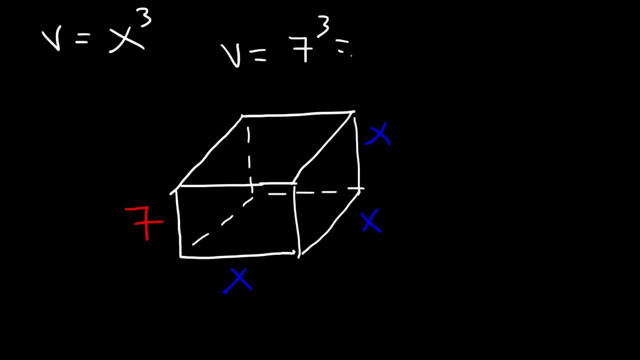 or 7 times 7 times 7.. 7 to the third power is 343.. So if this was 7 to the third power, it would be 7 to the third power. If this was 7 inches, this would be 343 cubic inches.